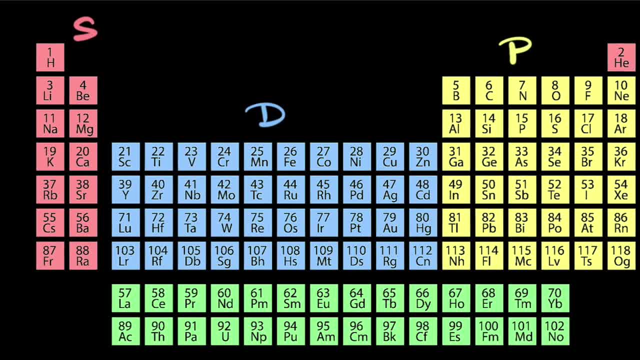 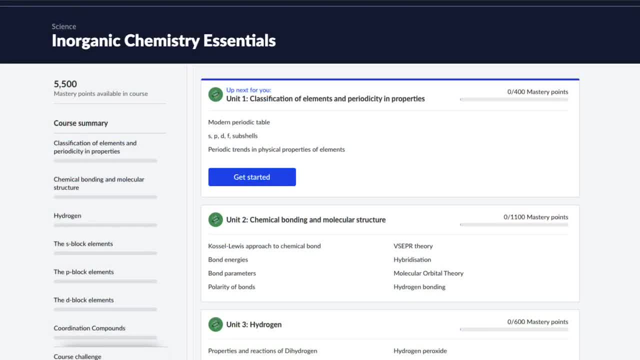 Would it be awesome to learn all of this and more, with pure logic? If your answer is yes, then I'll see you inside. This course covers all the essential topics of Class 11th and 12th CBC in modern science and chemistry. If you have questions or would like to learn more, 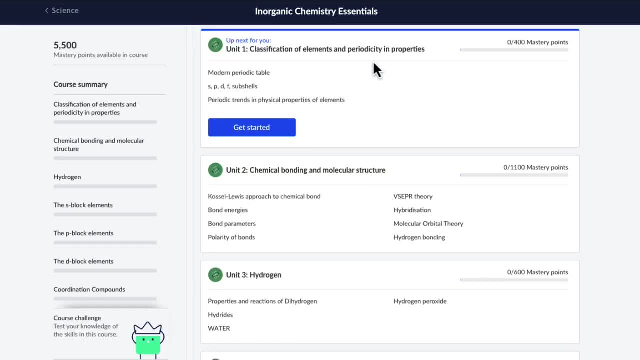 please leave them in the comment section below. Please subscribe to the channel and hit the bell icon to not miss new videos. If you have any questions or other questions, please post them in the comments below. inorganic chemistry and it starts with some basic ideas of your periodic table and chemical bonding. 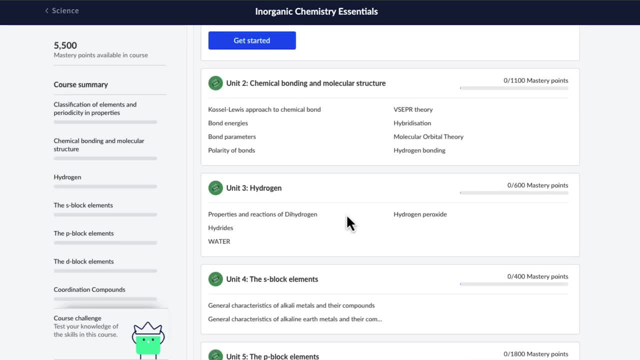 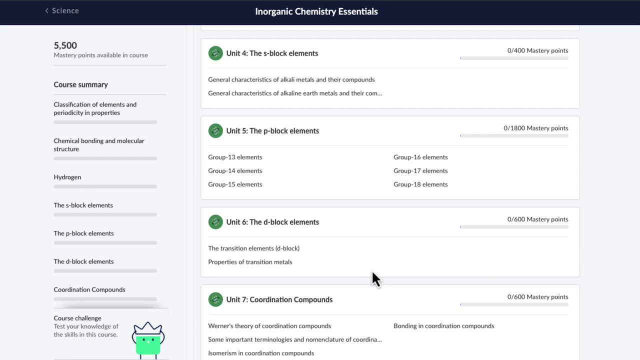 and then directly jumps into the elements: the hydrogen and the s block elements, the p block and then finally the d block and the coordination compounds, and the course mostly focuses on the common trends that you find within each block, within each group. this way you'll get a new 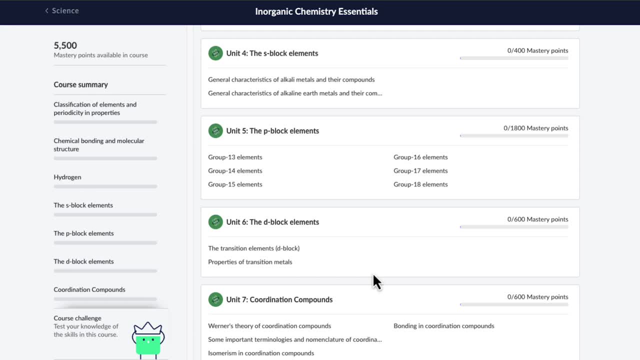 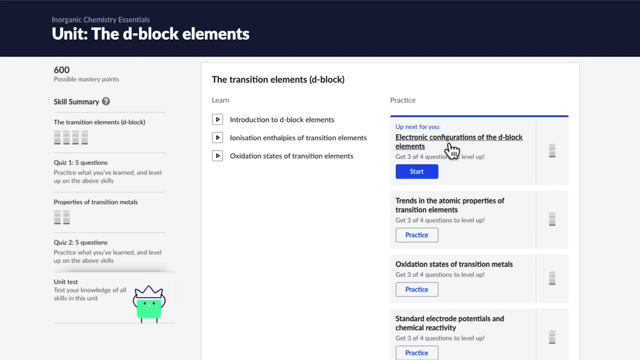 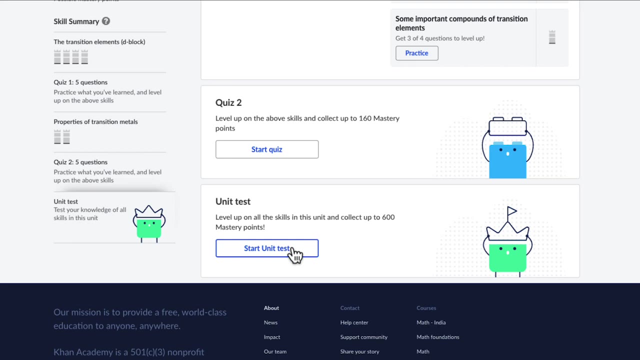 perspective on how to look at the entire periodic table to deepen your understanding of the elements. and, of course, inside each unit you have videos to give you instruction. then there are exercises where you can practice different questions to solidify your concepts, and then there are quizzes and unit tests which will jumble all the questions from different exercises to give you complete 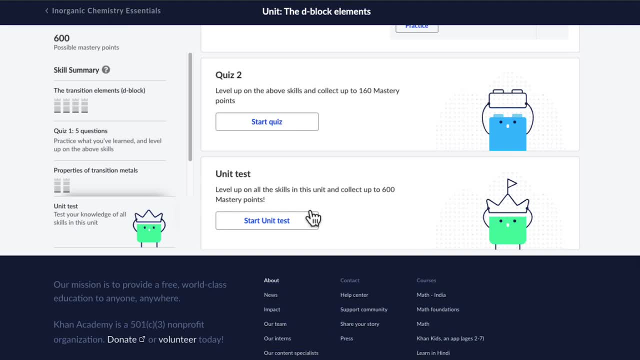 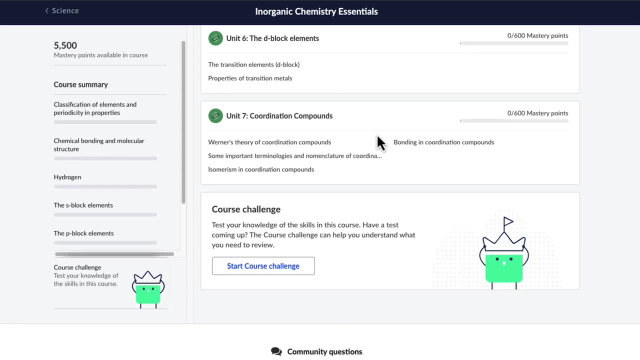 mastery over this entire unit. and then, once you have mastered all the units, you can take a course challenge which will jumble all the questions from all the different units to give you complete mastery over the entire course. so, yes, it's a pretty rigorous course to make. 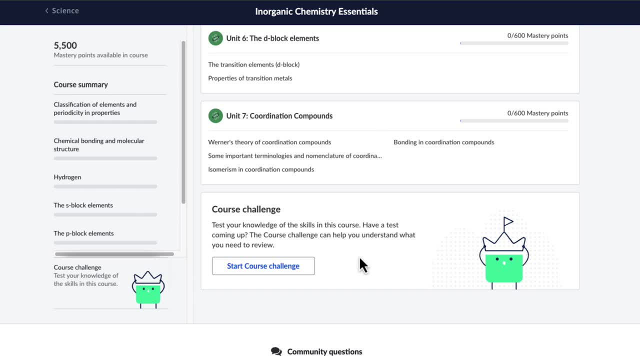 sure that you can solidify all the basic concepts and if you're excited, let's begin. 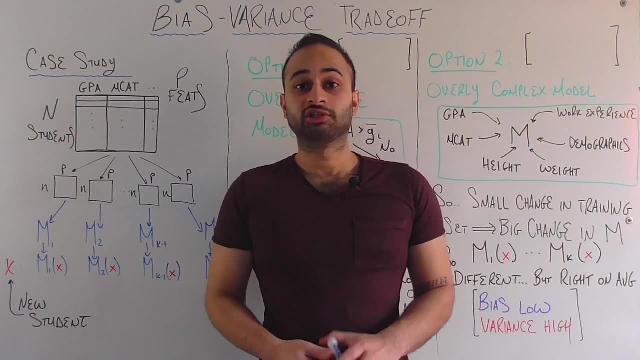 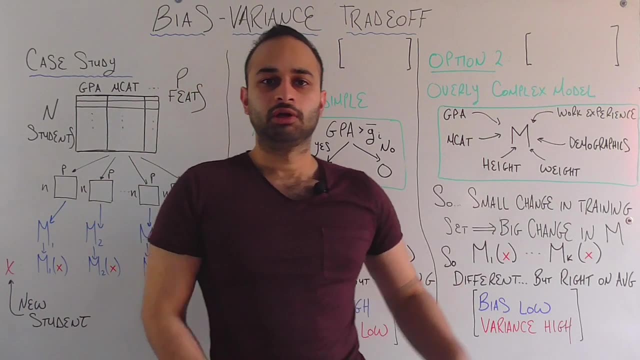 Hey everyone, welcome back. So today we're going to be talking about a very important but also often misunderstood concept in data science called the bias-variance trade-off. Now I really want to do a good job in this video, because it took me a while to fully understand the bias-variance.